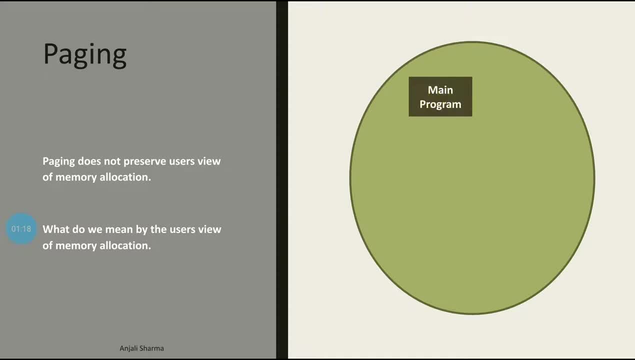 of your program as a whole, and it may be consist of a main function, some shared libraries, some stack that can be used for storing the variables and the intermediate results or even the recursive calls and certain predefined or user defined functions. You can also presume this as a C program, where a programmer first include the header files. they are one particular section, that is, the shared libraries. Then we have our main function. 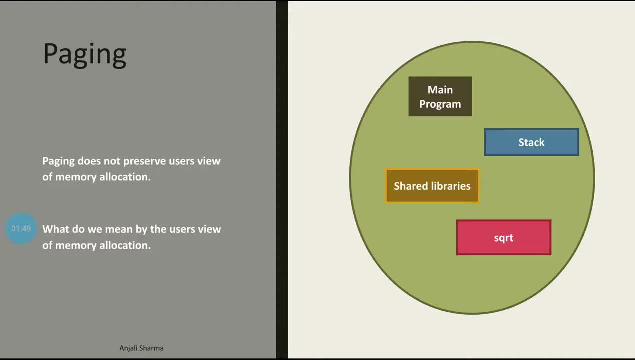 in which we initialize our variables and do our calculation or write our logics, so that may be the main program and the stacks. Similarly, we can also include some user defined functions or some predefined function, such as sqrd or a simple addition function that is user defined, So in paging the view or the memory, 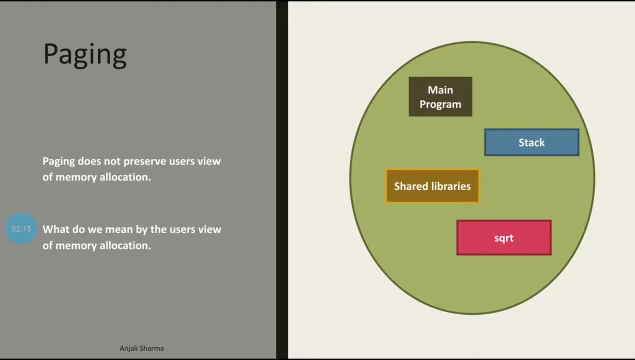 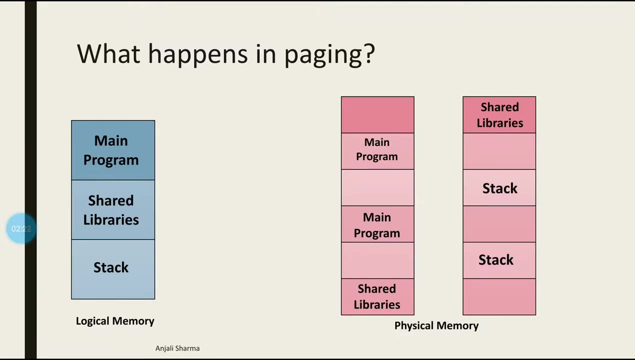 management do not look at a program as a collection of these components. So what paging does? So in paging, suppose we have a logical memory and logical memory has a single program having three components, namely the main program, the shared libraries and the stack. So what happens in paging These three components? 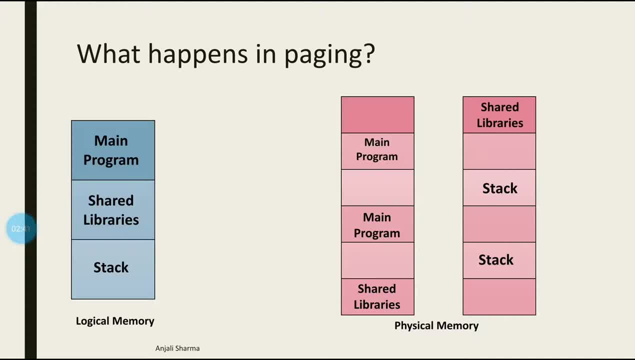 will be divided into equal size pages and then they will be transferred to the physical memory, into the free frames, right? So in basically what paging does, each portion of a program is divided into equal size pages and is stored in the physical memory's frames, right So? 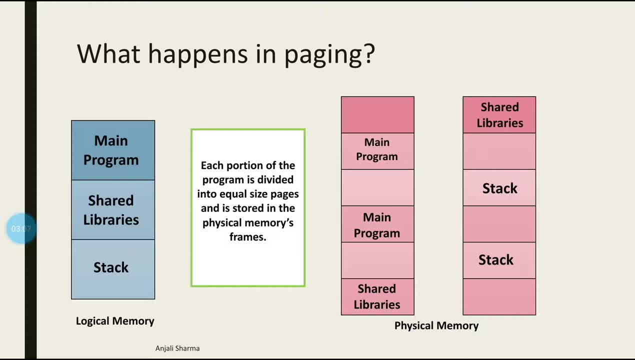 whatever were our components. these components are divided into equal size pages and they are kept in free frames. and again, address translation happens. But what happened on the user's perspective? what a user thinks? that the whole program is divided into only these three segments, that is, the main program, the libraries and 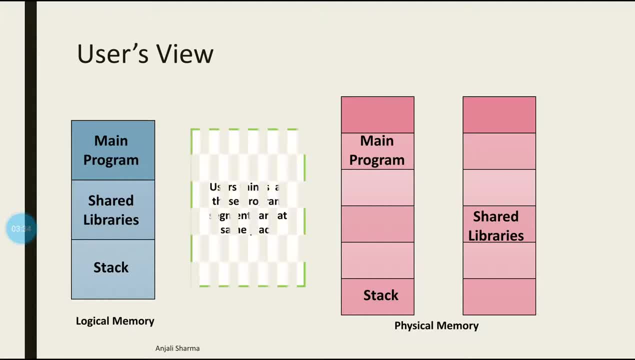 the stack. So, according to the user, he thinks that his main program is located completely at one location or one position in the physical memory. Similarly, the stack is divided into two segments and the stack or the shared libraries are there at one position. So the 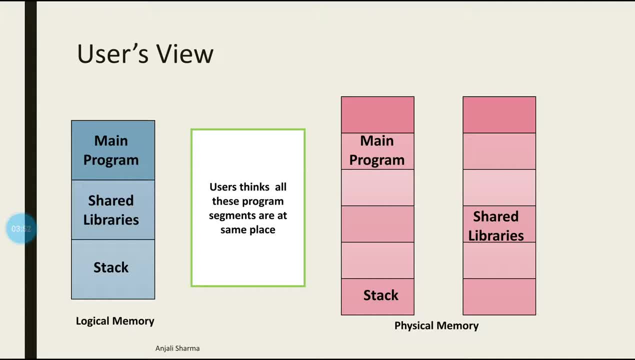 user thinks that all these program segments are placed at the same place. So now, what is the difference between the two and how? segmentation is somewhat beneficiary to your paging technique. See the address. translation becomes somewhat easier. So the implementation of segmentation as far as the paging hardware is concerned is a little bit easier, right? 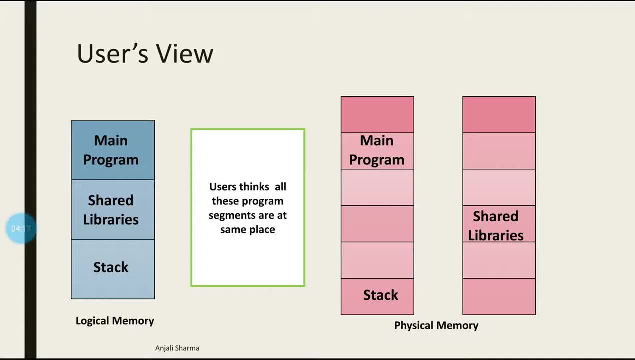 The paging address, translation is somewhat easier. The implementation of the paging hardware is. translation was a bit complicated one. Secondly, in segmentation, because the complete segment is placed in the physical memory, we keep the whole segment in the physical memory so it completely eradicates the internal fragmentation, Whereas in paging we have seen that because 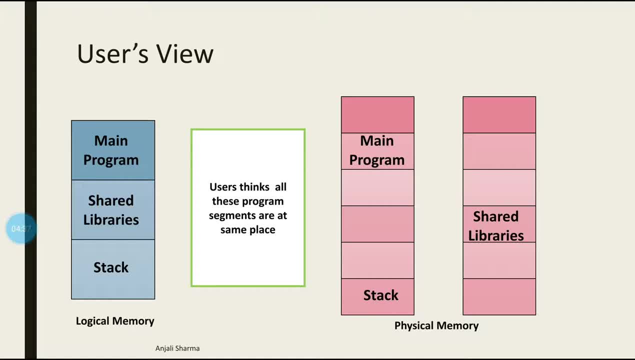 of the variable size of the last page. we divide the whole code in the page, so it is not the same. The last portion left we have is equal to the size of the page. For example, if we have a 12K program and we have made it in two K's, then we can have a total of 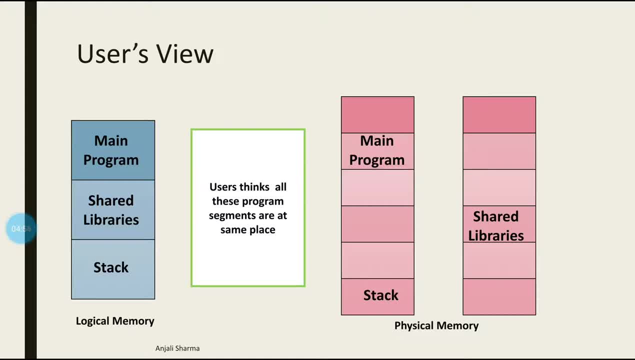 6 pages, Although if we have a 11K program then the last page will be of 1K. So that gets the internal fragmentation. but in segmentation internal fragmentation is completely eradicated. So it is somehow beneficiary to your paging technique because these external and internal 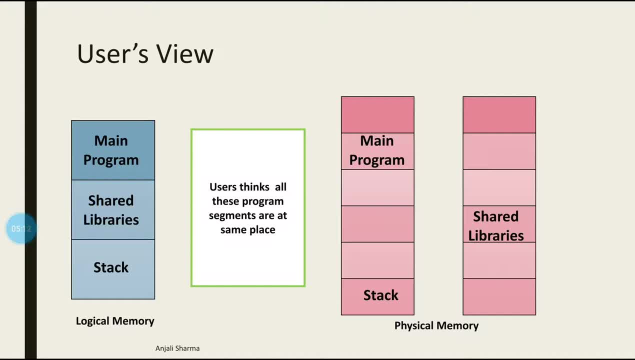 fragmentation is completely eradicated by your paging technique. So while in segmentation, internal fragmentation works on both. So that is why the concept of segmentation is a little bit better. or we can seeing in the upcoming lecture that we will be combining the both techniques in order to identify in 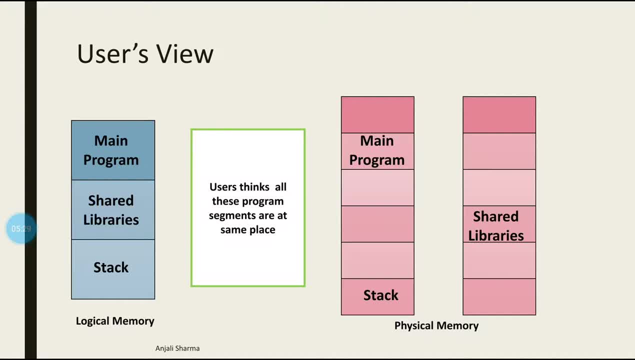 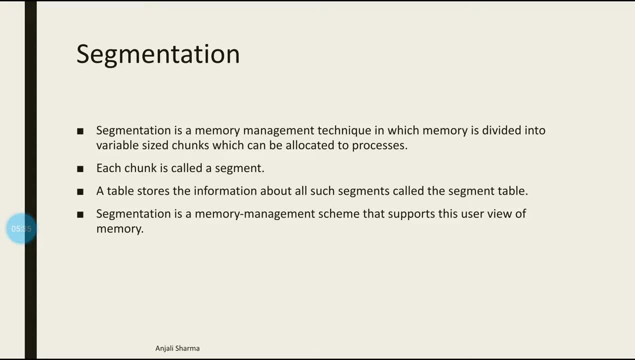 order to get the complete benefits, or the combined benefit of the both. So what segmentation is? it is a memory management technique in which memory is divided into variable size chunks which can be allocated to processes. Each chunk is called a segment. a table stores the information about all such segments and 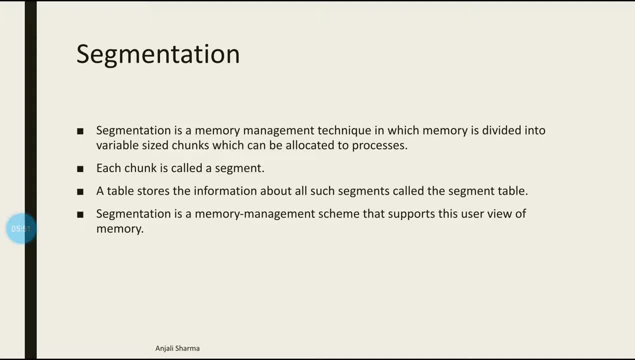 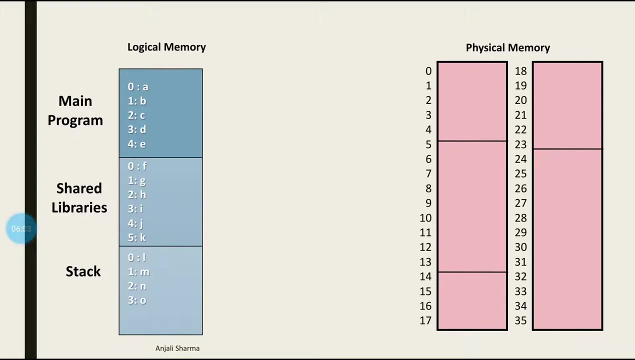 they are. that table is known as a segment table. Segmentation is a memory management scheme that supports the user's view of the memory. that we have already seen in the previous slides. So now let us see how memory segmentation address translation takes place. So the scenario says that we have a logical memory. suppose it is divided into three components. 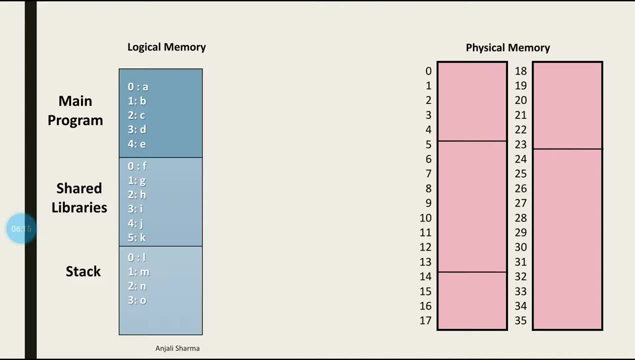 that is the main program, the shared libraries and the stack internally. you can see that the main program consists of five lines or five instructions: 0 to 4- that is the internal indexing and you can also call it as an offset- and ABCD are the instructions. similarly the 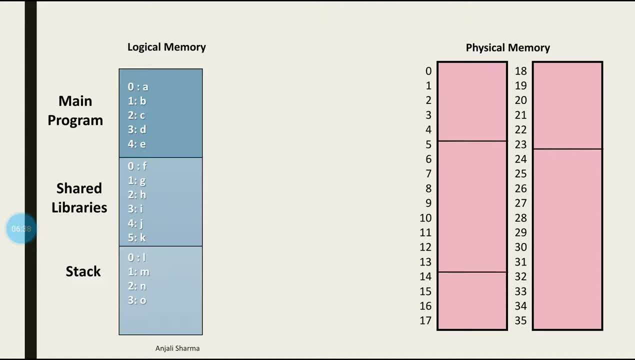 shared files and the stacks Are also having certain instructions right. So here in segmentation, it is completely evident that the main memory, or your logical memory basically, is consisting of three segments, that is, segment one, two and three respectively. So what happens when there is a need of executing the main program? it can be dynamically shifted. 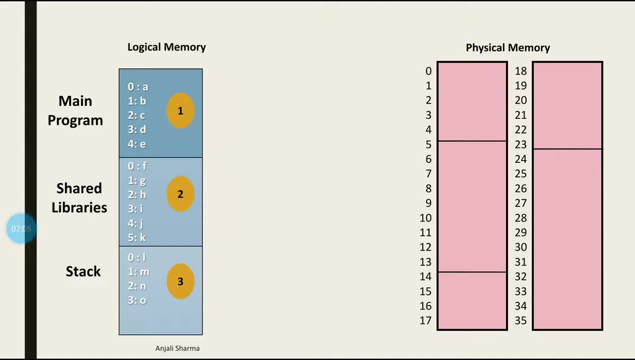 to a place in the physical memory That is Currently free or available. So whenever we have to execute the main program in the main memory, where can we keep it in the physical memory? whatever frame we have available, we can keep it dynamically, so always. 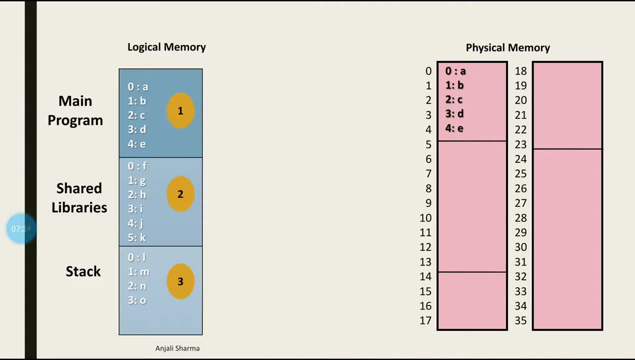 remember this. dynamic loading and linking is also very simple. or we can say that segmentation facilitates the working of dynamic loading and linking, which we have already read earlier. So now let us see how dynamic loading and linking works. Similarly, if we need shared libraries, then we can also dynamically keep them in physical. 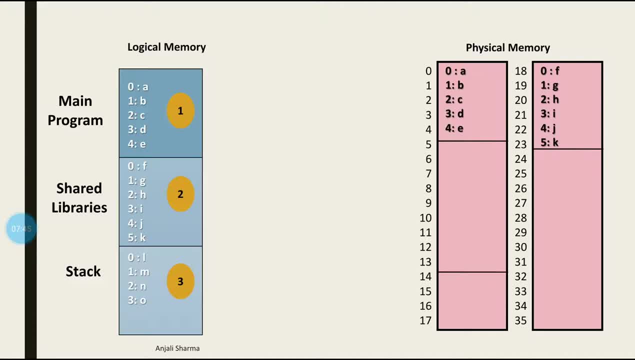 memory. That means, at the point of time at which we need to have the segment, we can take that segment and transfer it into physical memory. So here you have just seen that the three segments from the logical memory are now in physical memory. but again, the question that comes to us is of address translation. 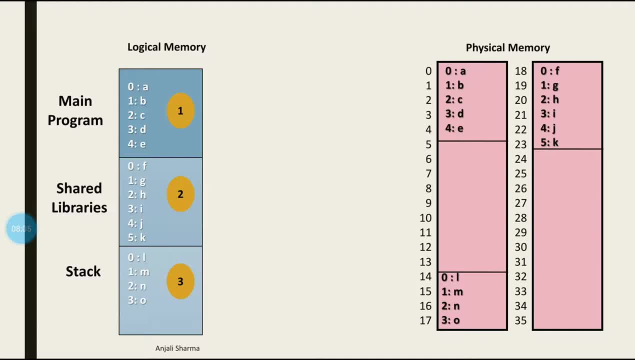 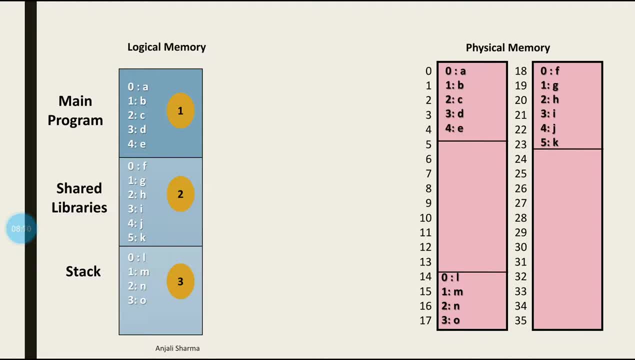 Same question. The CPU that generates a logical address does not have the knowledge of the physical address. So in order to know where the main program is or the shared library is in the physical memory, we require a mapping table, which is known as the segment table. 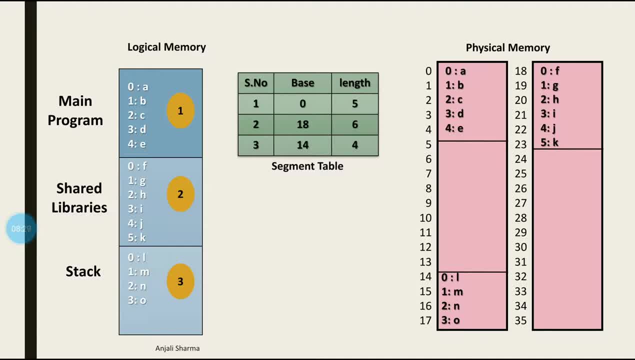 If it has been paging then it would have had the page table, but here you have the segment table. So in the segment table, the S number that is in the code which is the main program: jo hamara S number hai. that is the segment number. So you can see that there are three. 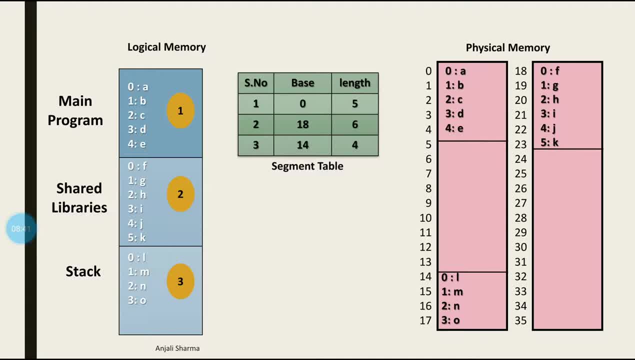 segments one, two and three. The second column is the base address. So, base address, kya hai Physical memory ke andar? just look at on the right hand side of the diagram, that is this pink portions, or the pink blocks of physical memory. It says that write the base. 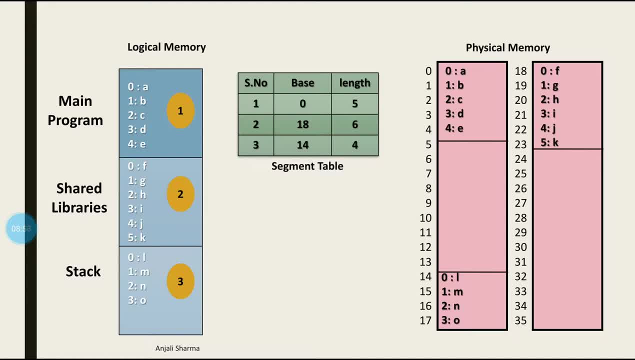 address Base address is the starting address right. So segment number one starts from address number zero. So you can see that it is starting from address number zero. Similarly, the segment number two, that is, your shared library, starts from the address number 18. 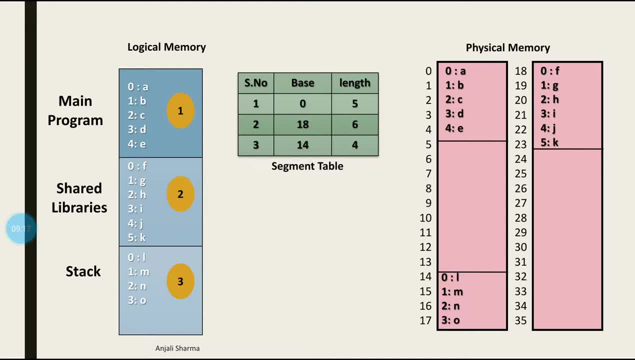 and the last segment, that is, segment number three, starts from address number 14.. So what is the base address? It is the starting address of your segment in the physical memory, because segment table acts as an index. So yaha par indexing kari gayi right Ab what? 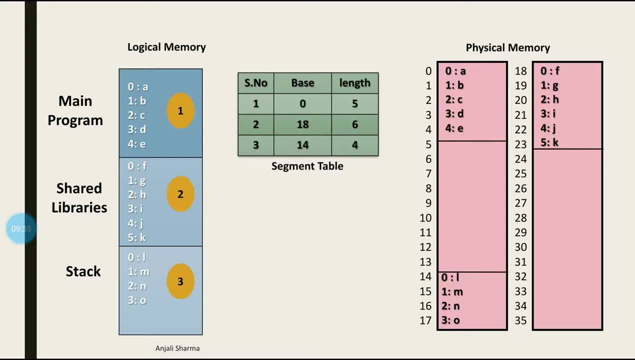 is the base address, It is the starting address of your segment in the physical memory. So what is the length? Length? it is the offset. Toh agar question mein kahin par offset likha ho ya length likha ho, toh you just don't get confused with it. So what length indicate? 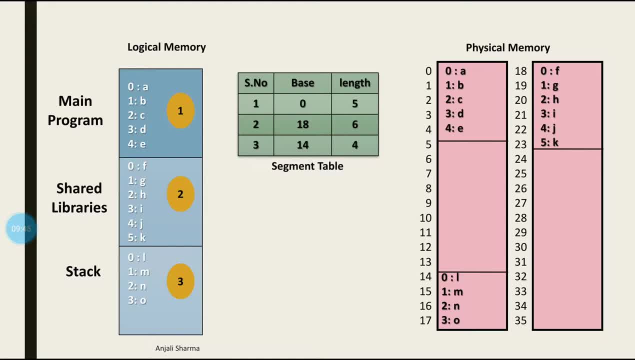 Length indicates ke zero se toh aapka segment man shuru hua, lekin jaata kahan tak hai. That means the size of the segment. So if you add five in zero, that means including zero. So zero, one, two, three, four, it equals to five. So four tak hama. 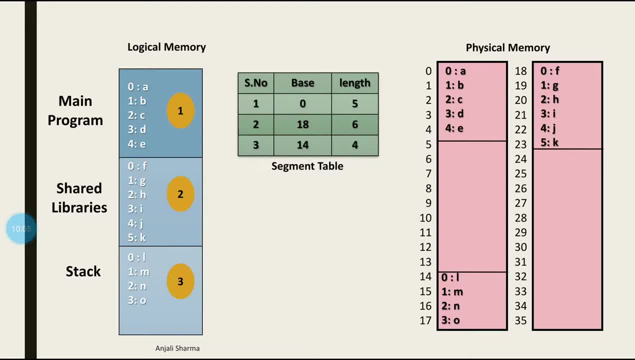 kiya hai, jo hamara main program hai. that is segment number one. it is spanning till four. Similarly, talking about the segment number two, that is eighteen, base address, aur wo chhe length tak jaata hai, Similarly the stack, it goes to length number four. 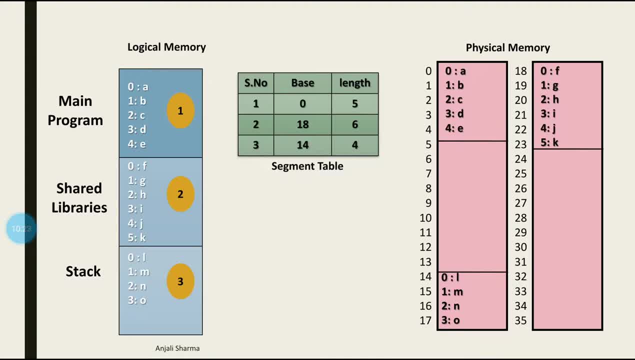 So what we did? we just had a indexing, or the mapping, with the help of segment table. So it consists of the segment number, the base and the length. Now what happens? Suppose what CPU wants to do: it wants to execute the third instruction of the main. 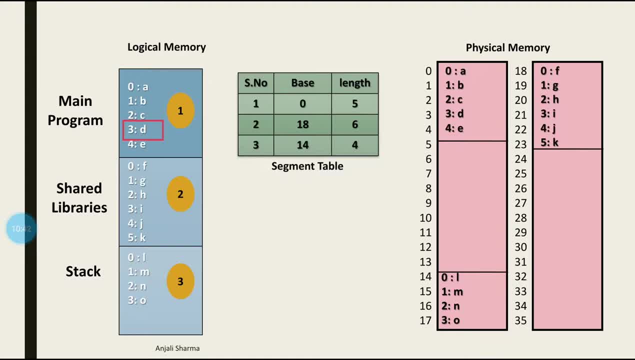 program. right. Toh ab CPU kya kahta hai, ki mere ko ye third instruction jo instruction number D hai, mujhe wo execute kara da hai. So now the issue is, ke CPU ke paas kaunsa. 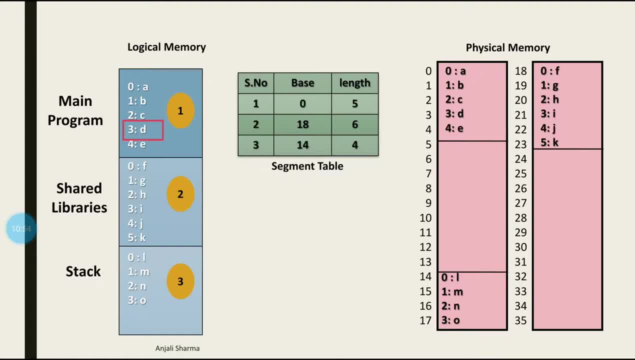 address hai Logical address. So in segmentation the logical address is a combination of the segment number and the offset. Toh, agar aap dihaan se dekhi, toh logical address is a combination of the segment number and the offset. So agar aap dihaan se dekhi toh logical. 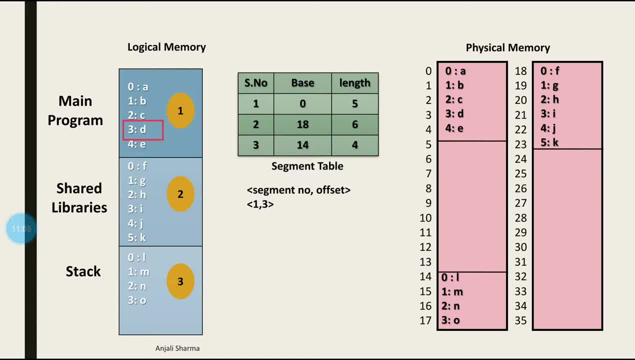 memory ke paas kya information hai Ke ye main program yaani ki segment number one ko belong karta hai? Ab diagram se bhi dekhi sakte hai? Oval me usse number padha chala ki ye mera. 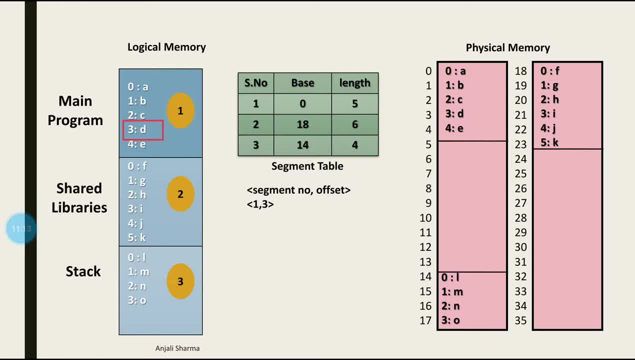 segment number one hai Plus usko internally malum hai ki ye mera third instruction hai. So the logical address will be a combination of segment number plus offset, So 1 comma 3.. Now the work is doing the address translation. This is the logical address and what we have. 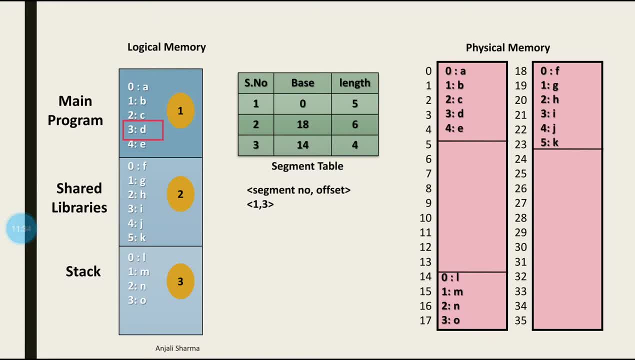 to do is to calculate The physical address. So we will be referring it to the segment table and we will be doing these three steps that are there on your screen. So with this 1 comma 3, we identify that it belongs to segment number one. So just follow that arrow and we get to the segment. 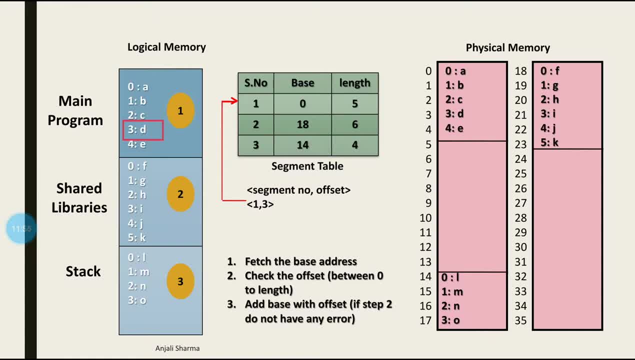 number one, Step number one says that: fetch the base address. So the base address is zero. So we identify that the base address is zero. So we identify that the base address is zero, So we identify that it belongs to this particular block. that is starting from. 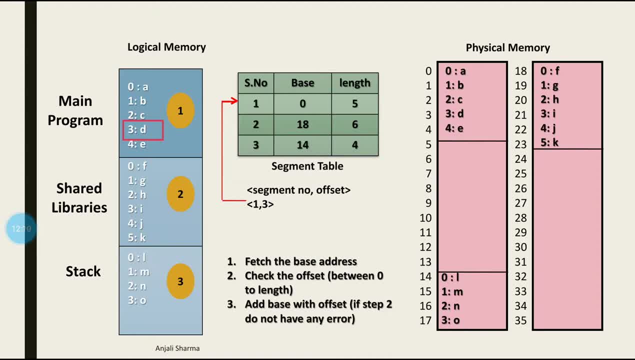 the address zero Right. The second thing says, step number two: check the offset that it should lie between zero to the length. See yahan par aap se kaha gaya ki pehle segment ka, step number three, execute. kariye Aap segment table pe gaye Aap ne padha kara ki wo kahan. 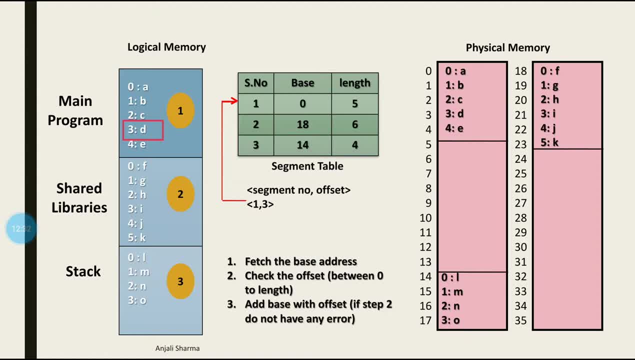 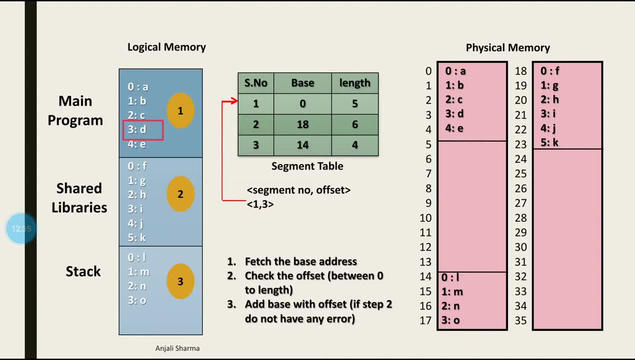 the offset on this single flat dennome. You have to pull out the offset of this single flat from the WiFi and from the connection to the Corda For that purpose. this grid here goes fromwn to the disk notch bar. So we are putting on parallel and then we are animating. 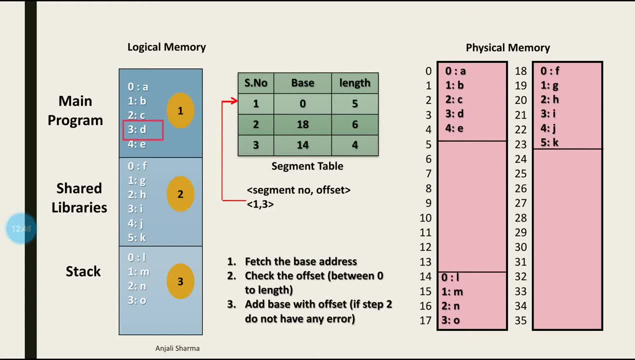 the offset in front of the grid as well. Alright, So that is the offset of the grid that we want to integrate for show. So we are succeed in putting off set ofuğколja. settings. aap kwala So reverse frontura. ha Highness, mean that there are errors. This butter has been. 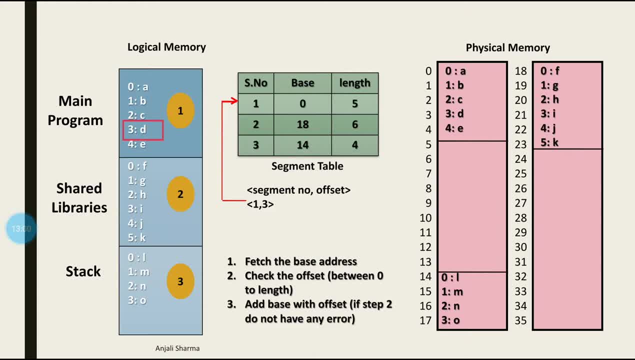 been done, but then the person also generated a trap. so it isdes ries ngau betne NEke to ten to do that what it has been done. 3 ko 5 jo ki uski length hai usse compare karwana hai toh it should be between 0 to length ya. toh wo length ke barabar ho ya usse thoda kam. 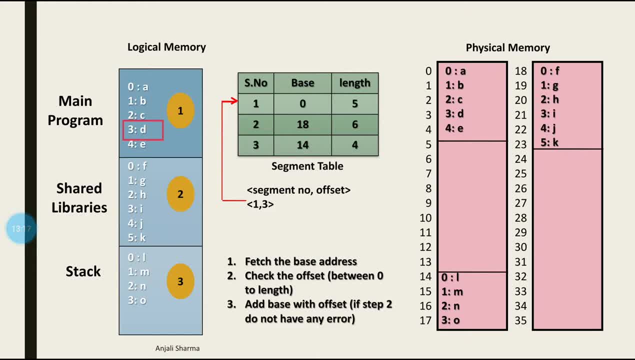 ho tabhi wo valid address hai, right? so the second step says that, whether you are accessing the correct instruction or not, wo address exist, bhi karta hai or nahi. so the second step is checking that particular thing. now, if the second step gets corrected, then add: 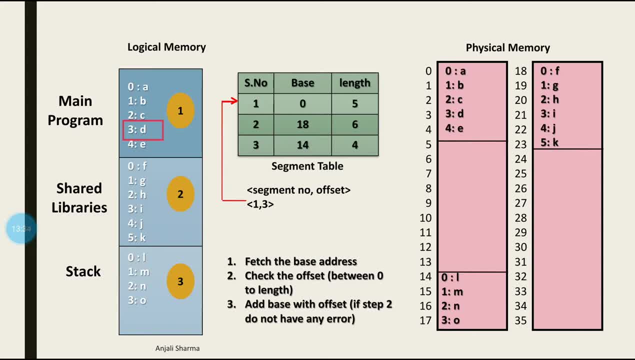 the offset to the base address. so what you have to do, you have to take the base address, that is 0, and just add 3 to it, right? so the answer come out to 3. that means it is clear that agar aap 0 ke anda 3 add karte hain, toh aap 3 par pahot jaate hain, right? so it is. 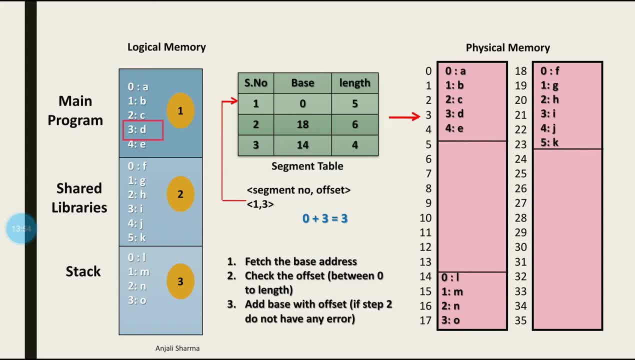 the same address that is being generated by the address logical address. so these three steps are very important and with the help of these three steps only we are going to do the numericals of segmentation. so that is how the address translation is done. the last step is adding the base with the offset and you are getting. 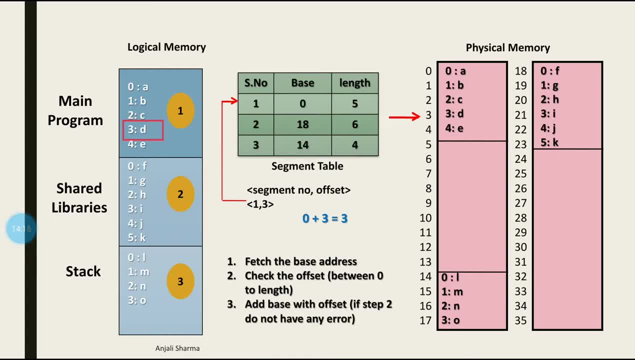 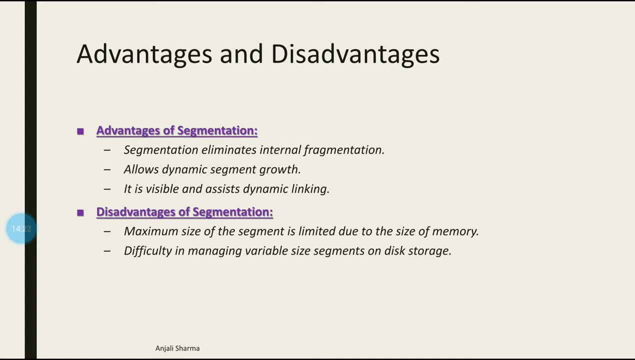 the address. so that is the address translation in segmentation and it is a very important topic. now coming to the advantages and disadvantages of segmentation. advantages of segmentation are the following: one is segmentation: segmentation eliminates internal fragmentation that i have discussed. it allows dynamic segment growth. it is visible and assist dynamic linking all. 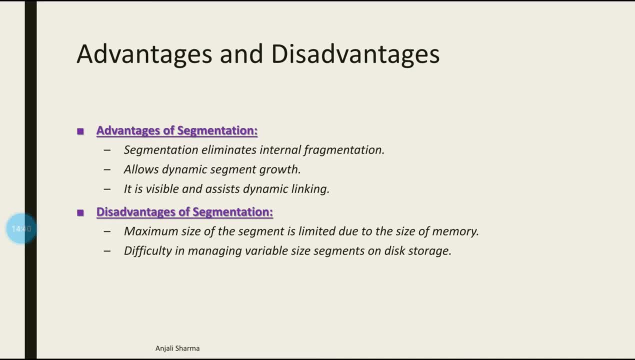 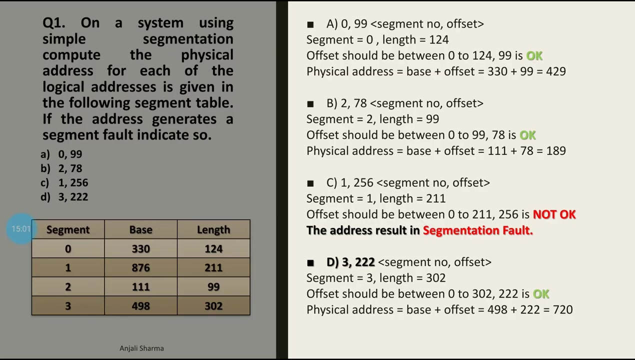 these things i have already covered. disadvantages of segmentation: the maximum size of the segment is limited due to the limited size of main memory. difficulty in managing variable size segments on disk storage. so these are certain advantages and disadvantages of segmentation and you can learn. now talking about the most important thing, that is, the numerical portion. 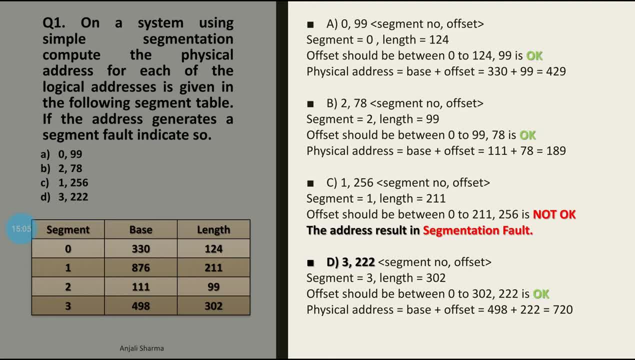 that comes in the examination. so if you have understood the address translation in segmentation, this numerical will be very easy to you. i am just reading the question and side by side i will be explaining how this question has been solved. on our system, using simple segmentation, compute the physical address for each of the logical addresses that is given in the following: 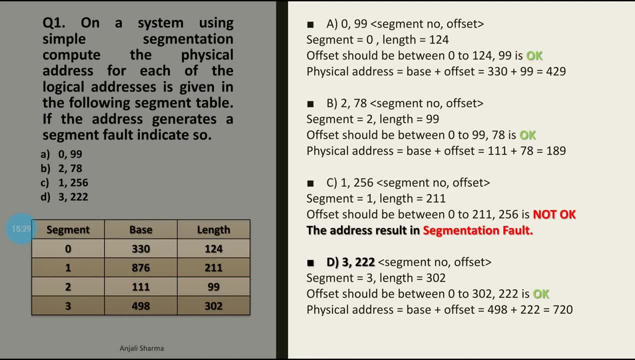 example, segment table. if the address generates a segment fall indicates so and there are certain data from a to d that is given and a segment table is given to you in the question. so what the question is basically asking here, these abcd, which are the parts given to you? 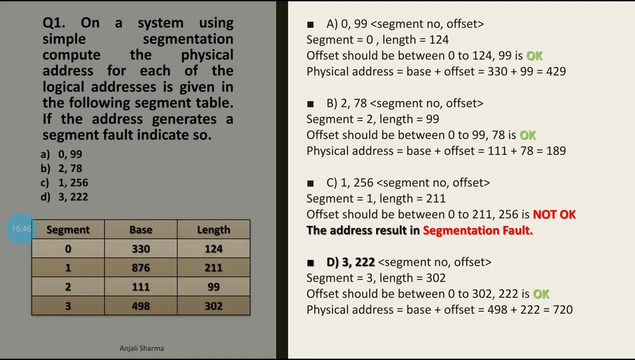 these are the logical addresses which we generate. that means if we look at the slide now, in the address translation, like in the first segment of 1 comma 3, it was told to execute the third instruction of the first segment. that is the logical part of the second segment. and now 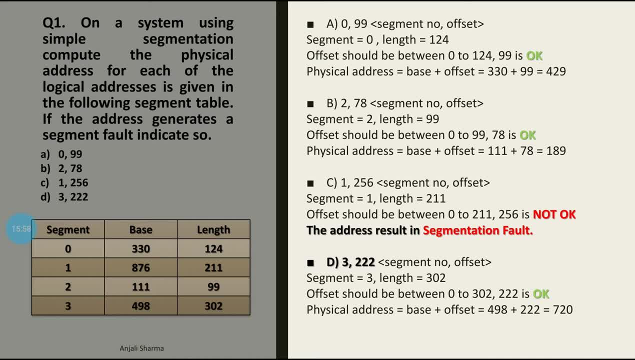 Similarly, the step number A says that the 99th instruction of the 0th segment has to be executed. So now you have to do the mapping similarly with the segment table. So let us see how it is done. So the A part says 0,99, which is the segment number and the offset. 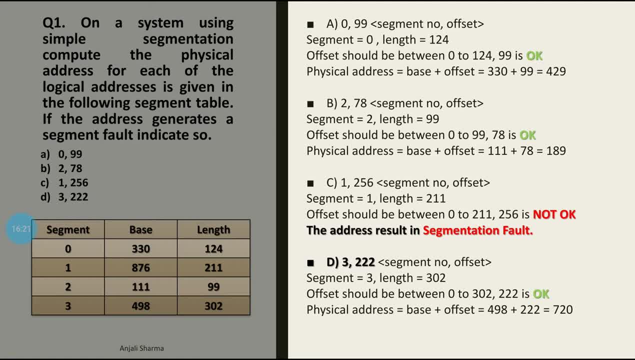 So here the segment is 0 and your offset is 99. So what you have is this logical address and through this you will go to the segment table. So when you go to 0th segment, this is the step number 1.. 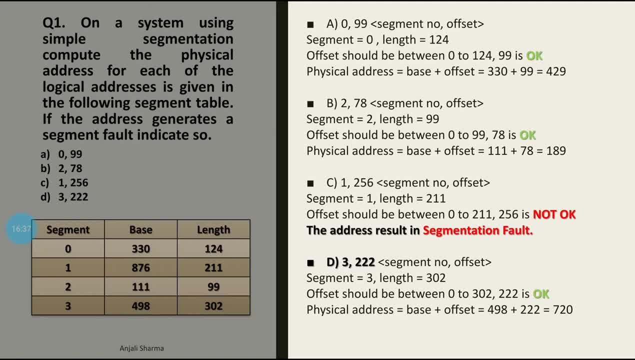 You go there and check whether segment 0 is available or not. So segment table has segment 0.. The next step is that you have to check the validity. Our second step was that we need to check whether the instruction, that is, the offset, given. 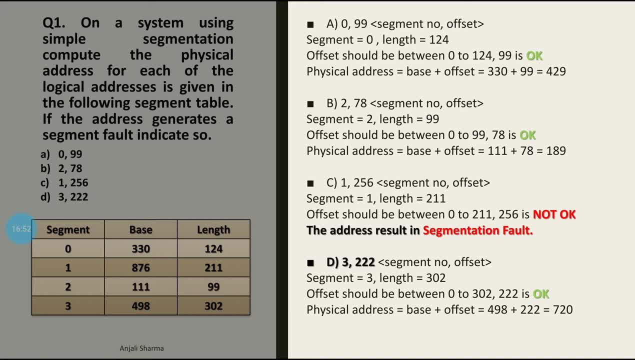 it should lie between the length range, right? So first of all we need the length. So we will see that the length of segment 0 is 124.. And the length given in the offset question is 99.. So it should always lie from 0 to length, that is, 0 to 122.. 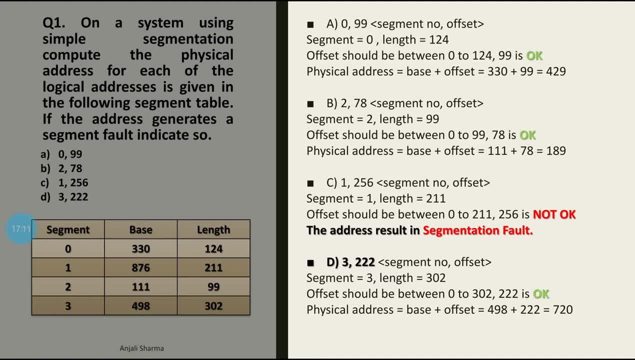 So 99 lies in this range. that means it is okay, We can execute that instruction. So finally, we will take its physical address. that is the addition of base with the offset. So the base value is 330.. 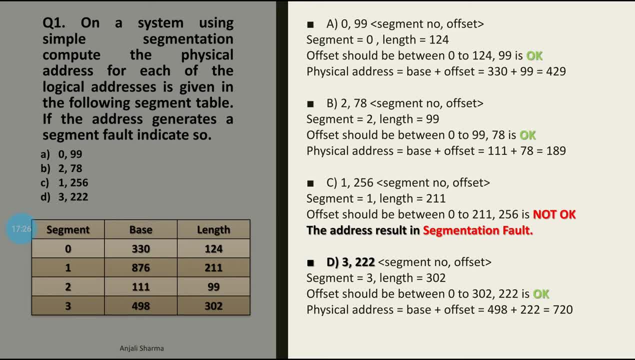 So that is again. we are fetching it from the segment table And just add 99 to it and 429 is the physical address answer. Similarly for second one, that is, B part, which has segment 2 and the offset is 78.. 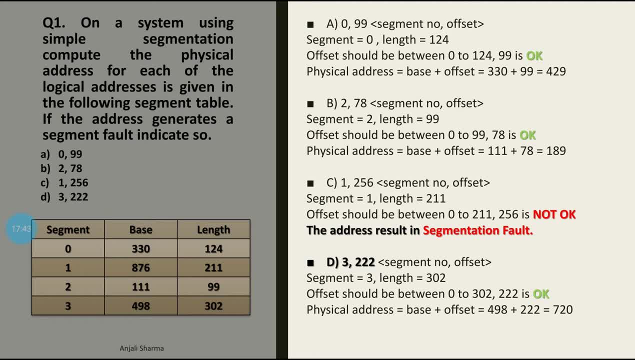 The segment value is 2 and the length of segment 2 is 99. So the offset should lie between 0 to 99 and 78 is a valid address. Therefore, adding the physical address For adding the base and the offset for the physical address, we get 111, that is the base address, plus 78, that is 189. 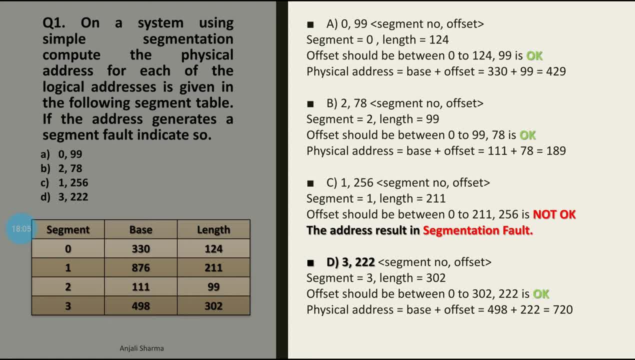 Now talking about this question, number C, The logical address which is given is 1256, right. That means we are talking about segment number 1 and the 256th instruction of segment number 1.. So the segment is 1 and the length of the segment is 211, right. 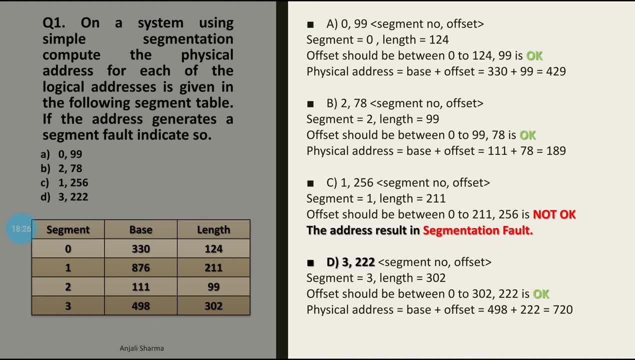 So the offset should lie between 0 to 211.. But it is evident that 256 is not okay because it is larger than 211.. So what? it means That we have 211 instructions in segment 1.. And you were told to execute 256th instruction. 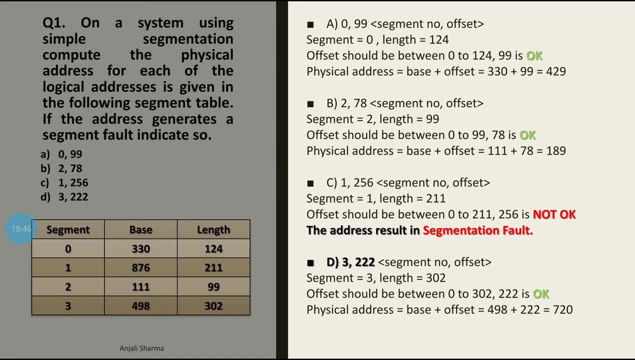 So it is not possible. So that is a segmentation fault. So what you have to mention is that this instruction cannot be executed. That is a segmentation fault. And similarly the D part can be done similarly. So that is the numerical that is basically asked in your examination. 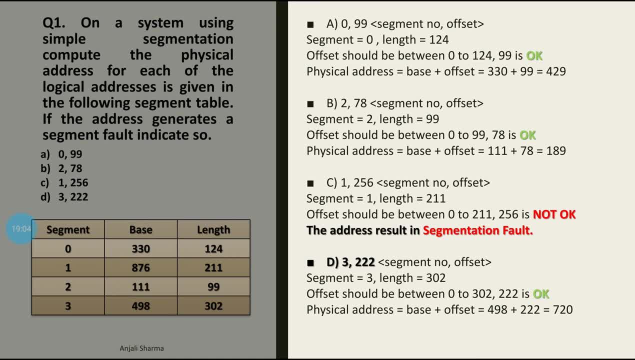 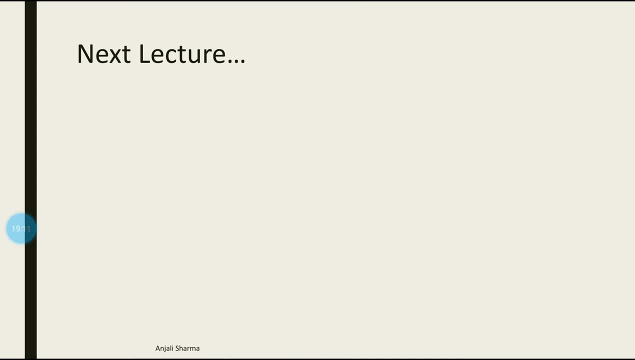 It is a very easy numerical, So if you understood the address translation, you can solve this particular question as well. So, coming up to the next lecture, we will be looking at a combined approach of paging and segmentation, which is page segmentation. 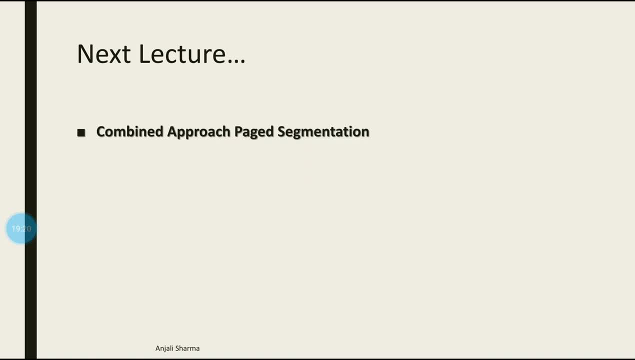 That is, we try to implement the advantages of both the techniques into one memory. So that is, we try to implement the advantages of both the techniques into one memory. So that is, we try to implement the advantages of both the techniques into one memory.